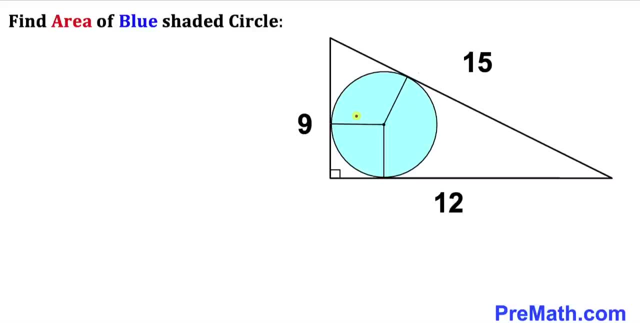 much nicer looking diagram where- let me go ahead and call these radii. i'm going to call this radius r, this radius r is the radius r r and this radius r as well. and now let's recall the circle theorem. according to this theorem, the angle between the radius and the tangent will always be exactly 90 degrees. so therefore, our 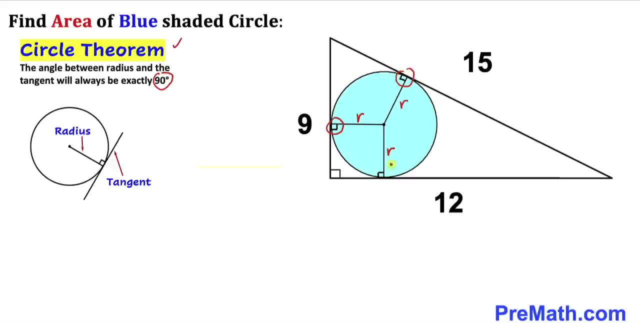 these angles are going to be 90 degrees each, and now we can see that this is radius r. so therefore this side length is going to be r as well, and likewise this length is going to be lowercase r as well, since the radius is r over here as well, and now we know that whole length is. 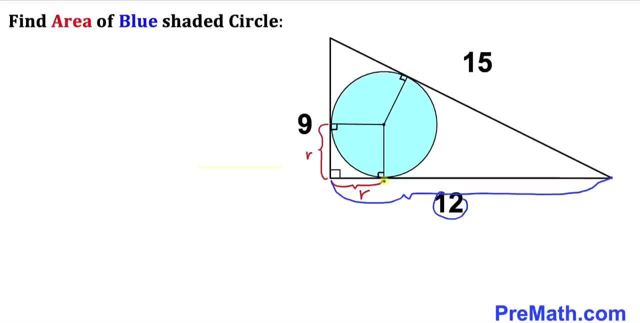 12. so therefore, this side length is going to be simply 12 minus r. so therefore, this side length is going to be 12 minus r, and on this side, our, this whole length is 9 units. so therefore this side length is going to be 9 minus r. and now let's recall two tangent theorem. according to this theorem, if two tangent 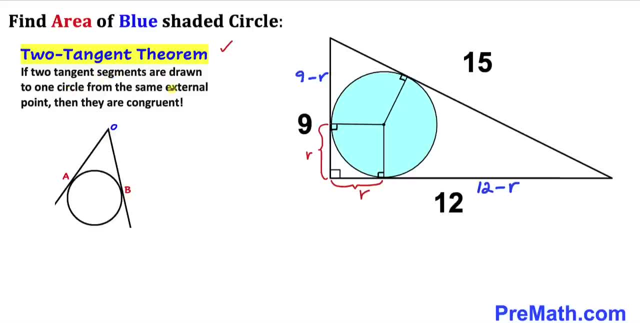 segments are drawn to one circle from the same external point, then they are congruent, as you can see in this theorem diagram. so therefore, we can see that this line segment is congruent to this one and likewise- let's focus on our this given problem. so that means this line segment is going to be congruent. 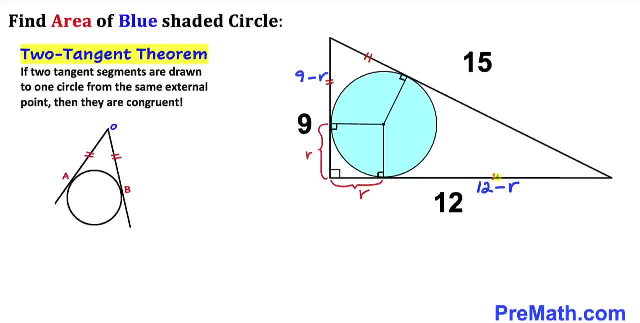 to this one and this line segment is going to be congruent to this one. so therefore, if this side length is 12 minus r and they are congruent, so therefore this side length is going to be 12 minus r as well. and now we know that this side length is 12 minus r and this whole side length is 15. so therefore this: 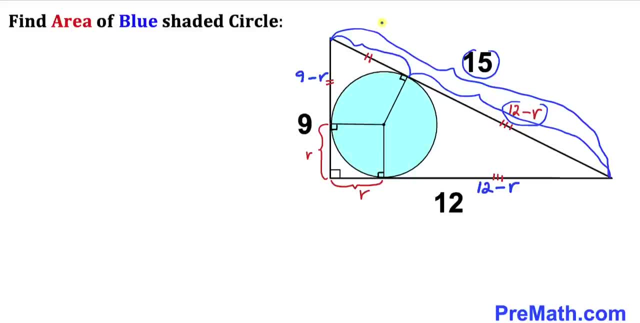 side length is going to be simply 15 minus r. so, therefore, this side length is going to be 12 minus r and this whole side length is going to be 15 minus r, and this whole side length is going to be 12 minus r. let's go ahead and simplify this thing. let's go ahead and distribute this thing. that's going to. 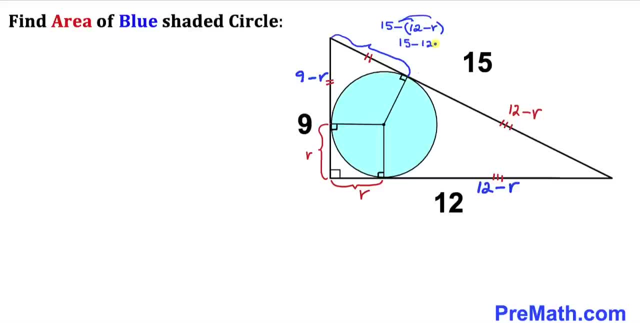 give us 15 minus 12 plus r, and if we simplify this, that's going to give us 3 plus r. so that means this side length is going to be 3 plus r, and now we can see that this side length is congruent to this side length. this side length is 9 minus r and this is 3 plus r. 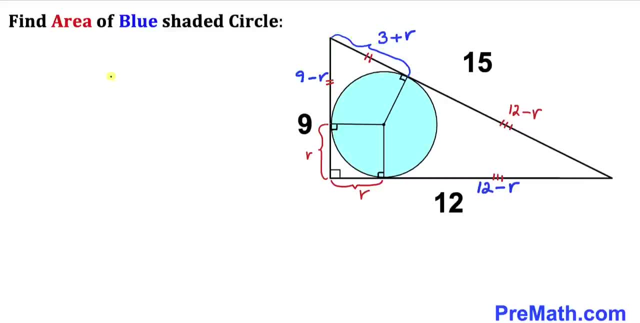 so therefore we can equate them now. so therefore i can write 9 minus r, equal to this other side. length, 3 plus r. let me go ahead and move this 3 on the left hand side and negative r on the right hand side, so this is going to give us 9 minus 3, equals to r plus r. so therefore we got. 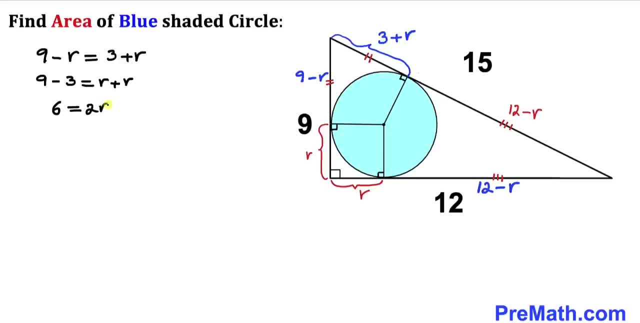 6 equals to 2r. let's divide both sides by 2, so therefore our radius r turns out to be 3 units. so therefore, our this radius turns out to be 3 units each. here's our final step. let's go ahead and calculate the area of this blue shaded. 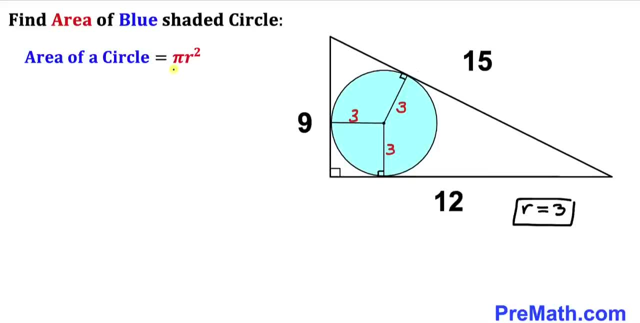 circle. and now let's recall the area of a circle. formula area equals to pi r square, where our r value we figured out equal to 3. so therefore the area of this blue shaded circle is going to be a pi times 3 whole square. so area turns out to be simply: 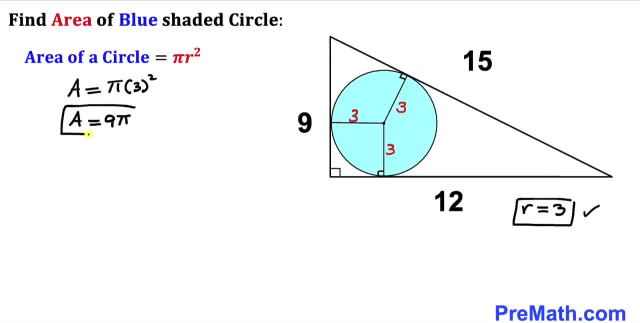 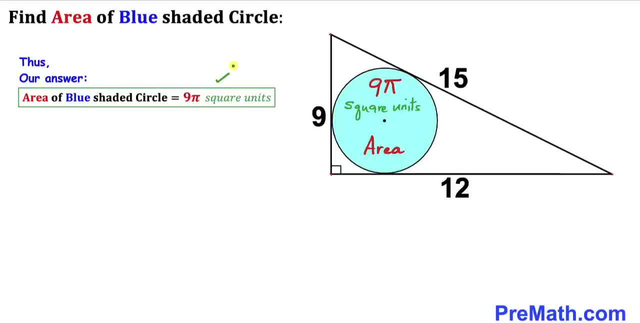 9 pi square units, so thus the area of this blue shaded circle turns out to be a 9 pi square units, or this is approximately equal to 28.3 square units, since pi value is approximately equal to 3.14. thanks for watching and please don't forget to subscribe to my channel for more exciting videos. bye you.